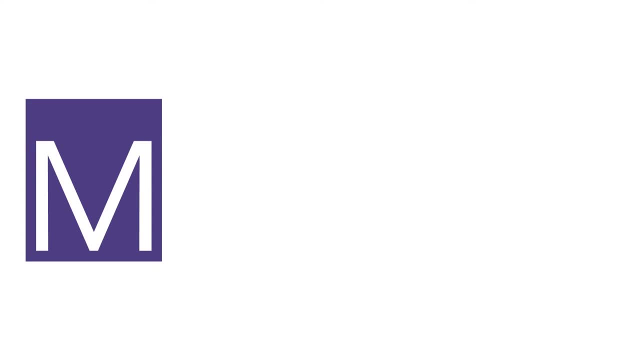 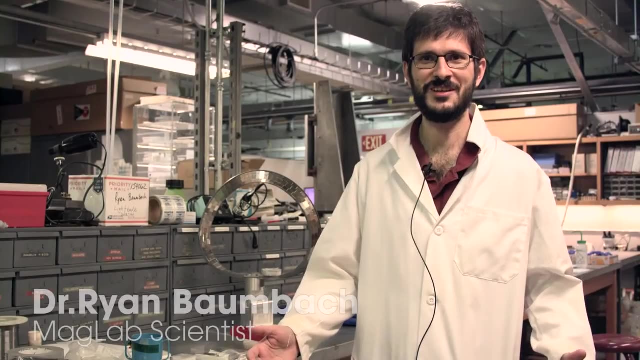 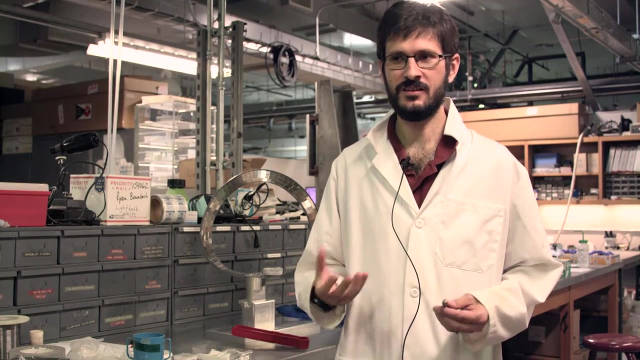 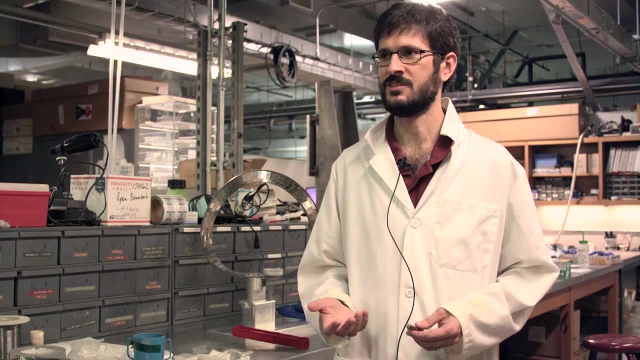 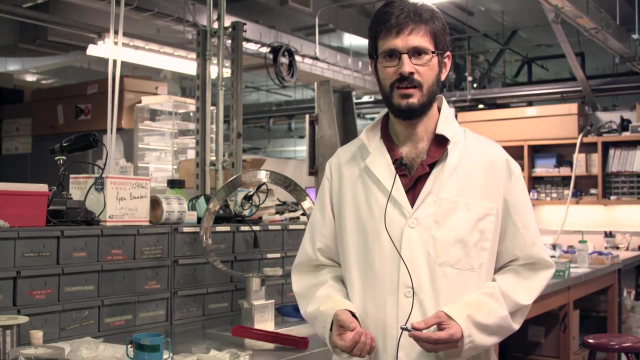 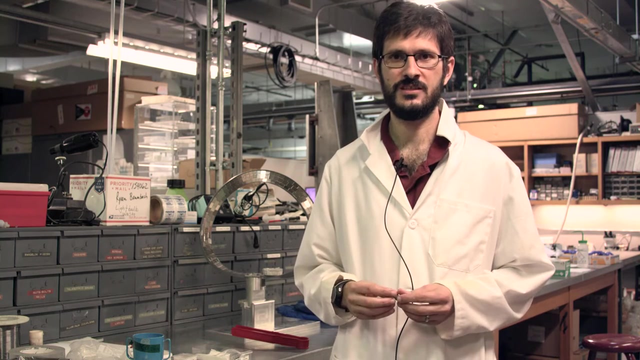 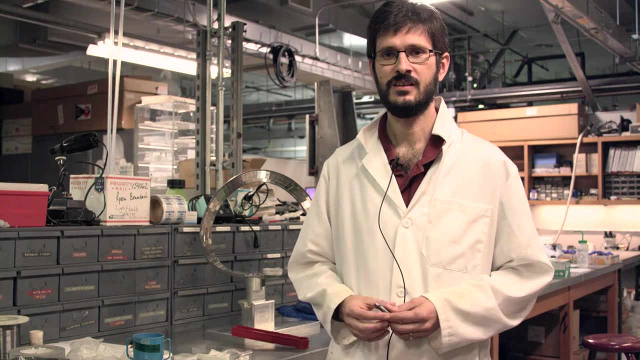 Welcome to the C-Wing of the Mag Lab. In this part of the Mag Lab, our work focuses not necessarily on experiments in high magnetic fields, but rather on developing the materials that we want to study in high magnetic fields, And in this group one of our main activities is not only developing new ways to grow crystalline materials, but also ways to grow very high quality specimens of materials that support very intriguing states of matter, like unconventional superconductivity, topological surface states, so on and so forth. 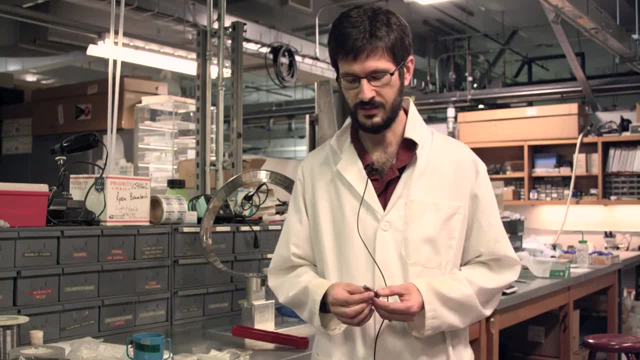 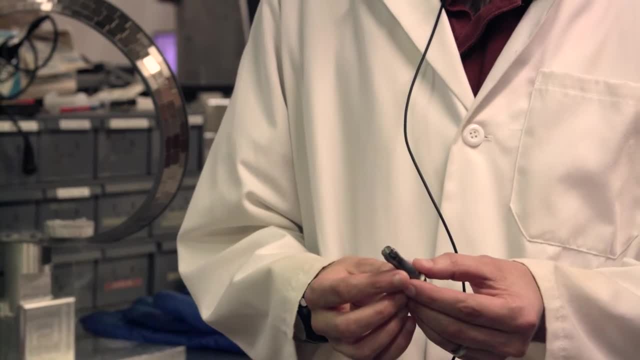 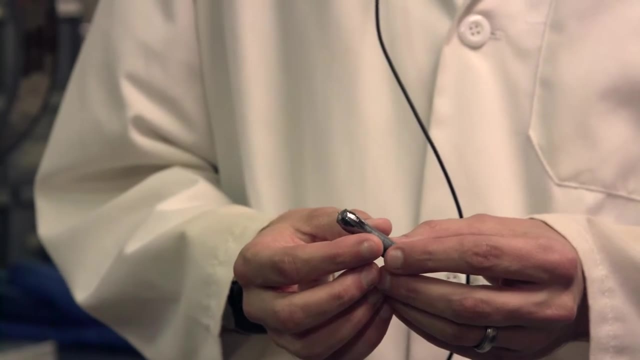 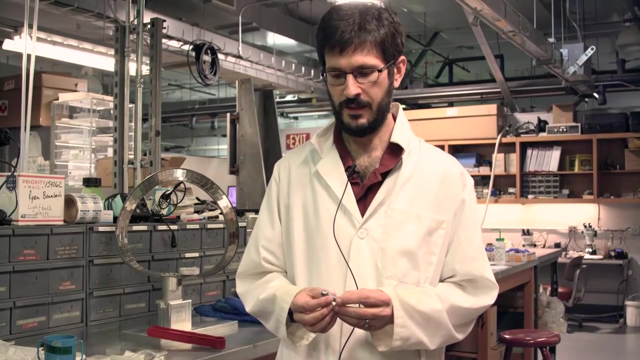 So the first thing that I want to show is a crystal of silicon, Which we grew in an apparatus that was built here by graduate students and undergraduate students. When you start with a piece of silicon just out of the bottle, it's typically in a polycrystalline form, which means that the atoms are, on a small scale, arranged in a regular periodic lattice, so they're crystalline. 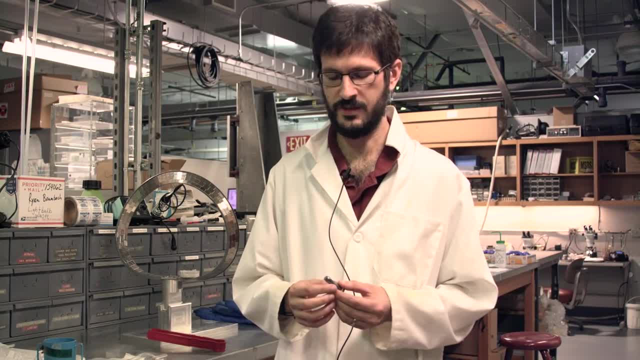 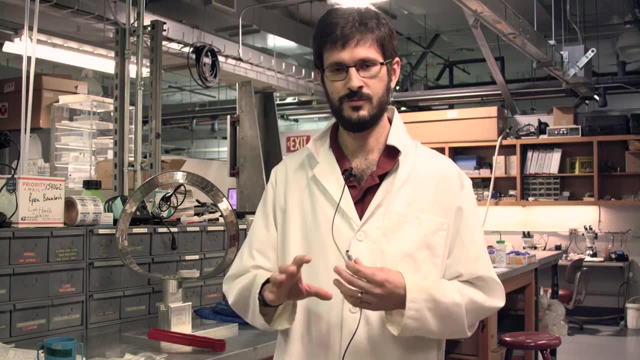 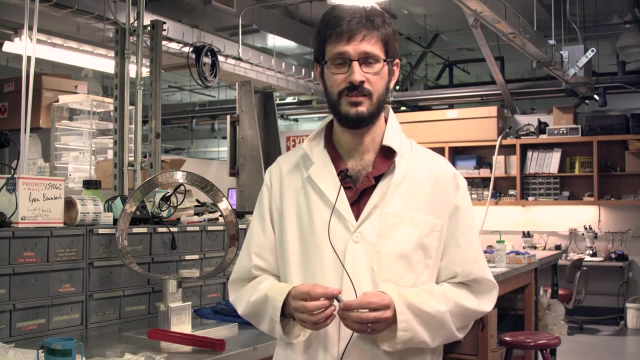 But on a larger scale. those little grains are randomly oriented with respect to each other. In a single crystal of the sort that we show here, those randomly oriented grains have been lined up perfectly. And from the point of view of an individual atom, the crystalline lattice goes on to infinity. 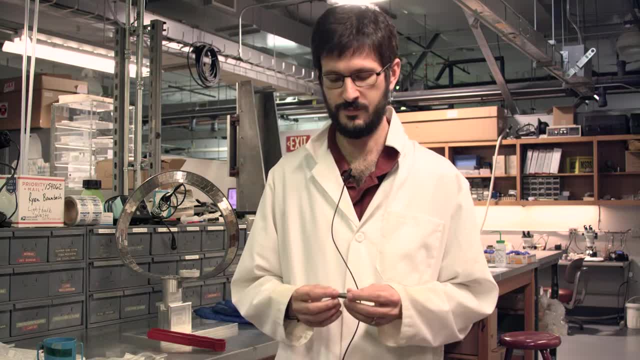 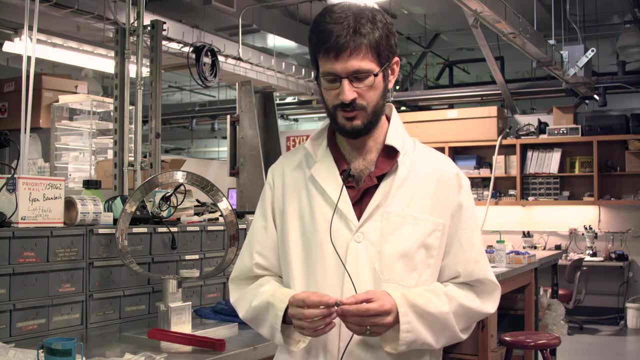 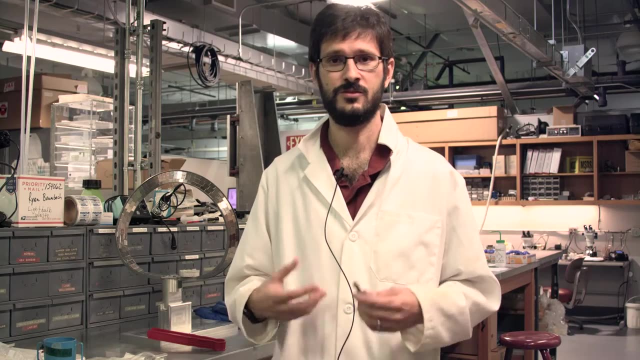 And this is exactly the type of thing that we want to study, because once we arrange atoms into this very periodic type of lattice, it's possible to really understand their fundamental electronic, or in other words their fundamental magnetic properties. So we want to study what are our materials magnetic or superconducting properties? 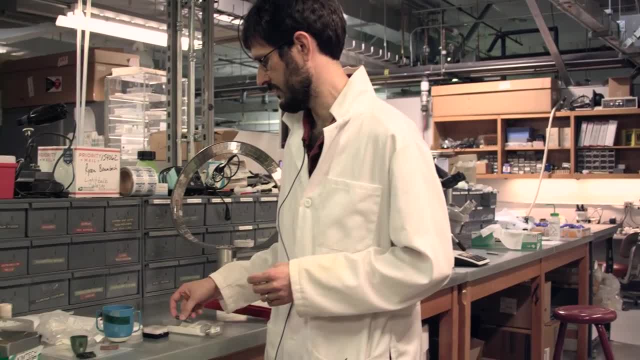 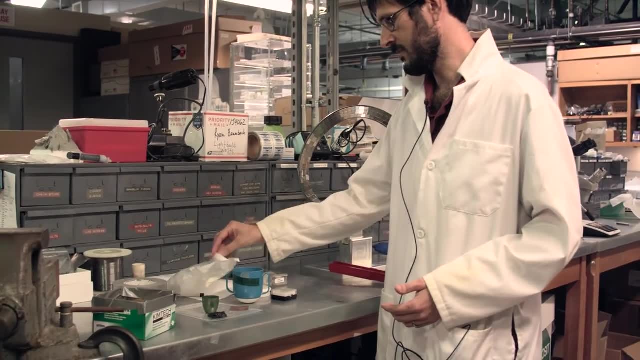 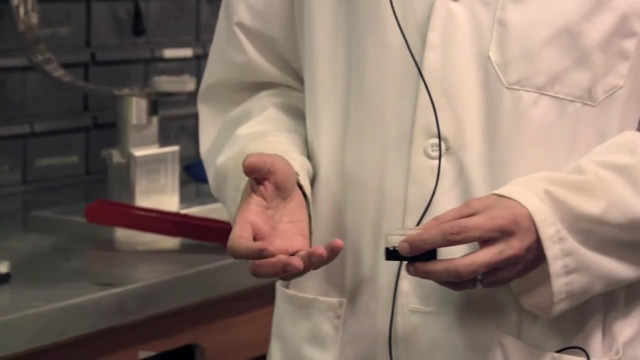 So this is a good example of the sorts of efforts that we make at growing nice crystalline materials. Now, not all materials are as simple as silicon, And keep in mind that silicon underpins a lot of technologies that we have these days. But now we're trying to study more complicated electronic states. 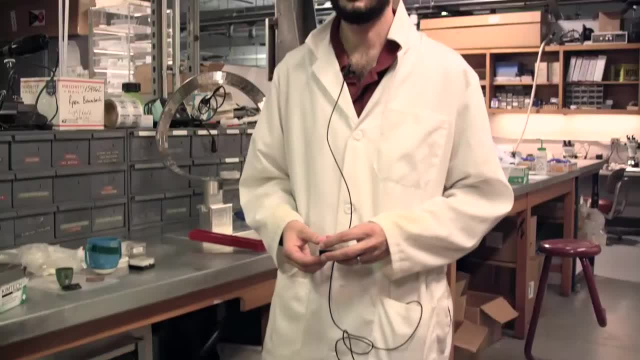 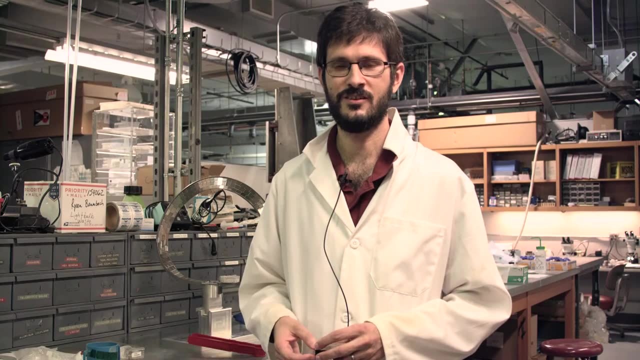 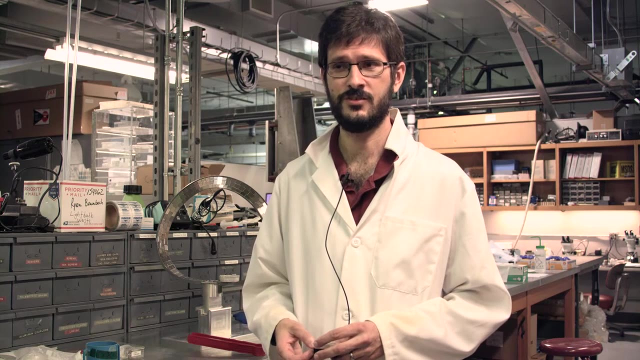 And sometimes it happens that they're not as simple as silicon. And sometimes it happens that when electrons get together in just the right way, they begin to behave in ways that are not very typical of individual electrons And that you might call a correlated electron state. 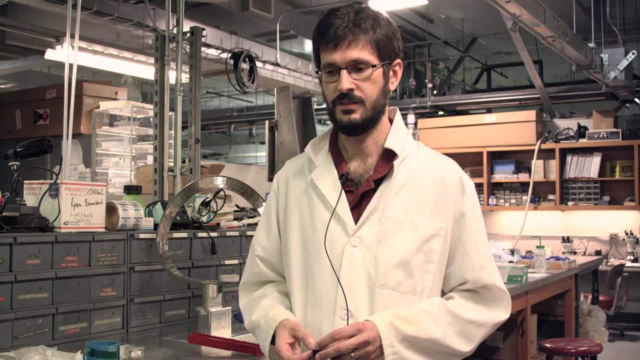 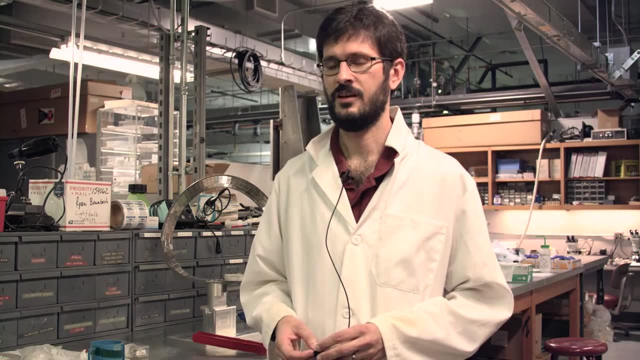 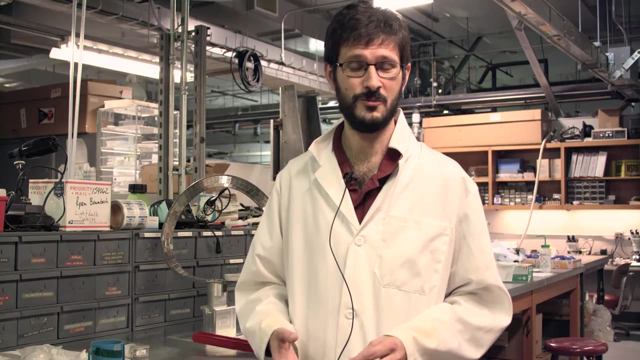 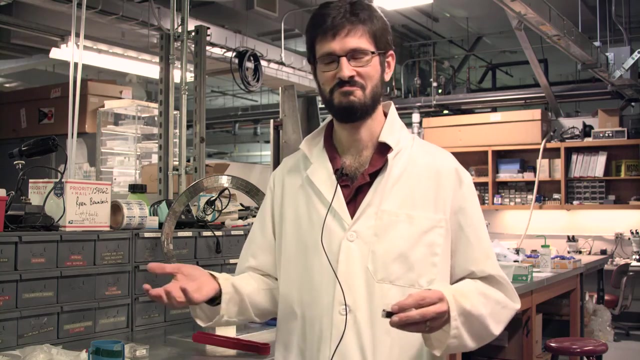 We'll typically see that well in this lab we like to study that type of physics in materials that have D electrons like iron Or F electrons like cerium- And probably people are familiar with cerium or other members of the lanthanide series because that's the sort of stuff that's in a lighter for lighting things on fire. 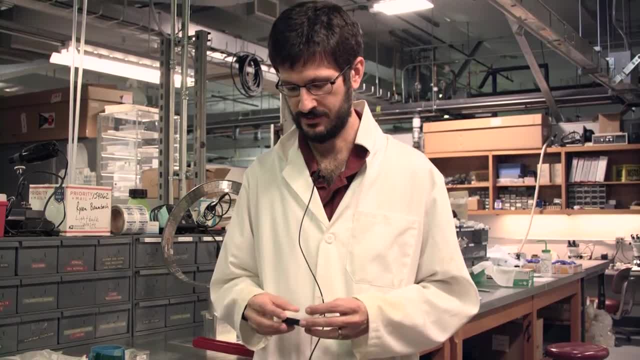 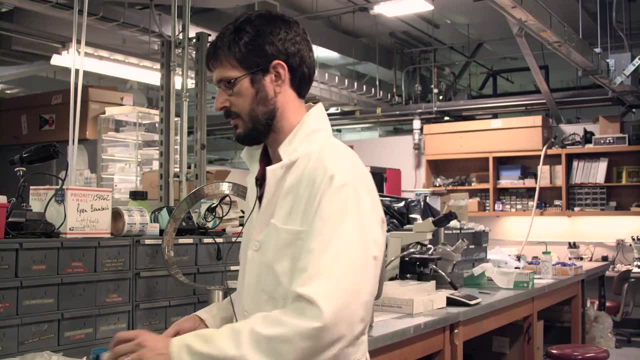 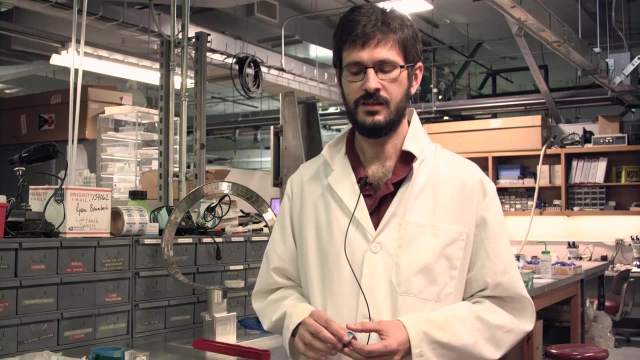 Okay, so those elements have very interesting properties. One subset of behaviors that we're very interested in is superconductivity. Superconductivity has been known for just over 100 years now. There's two general classes of superconductors, called conventional and unconventional. 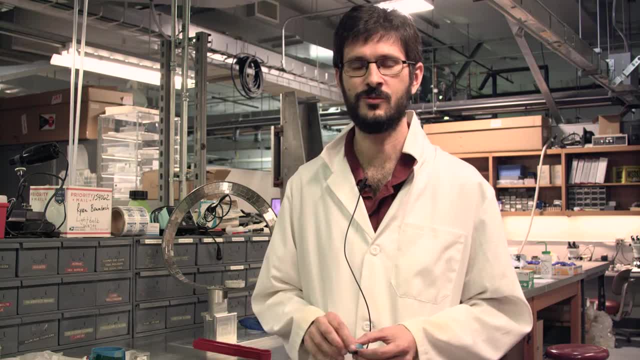 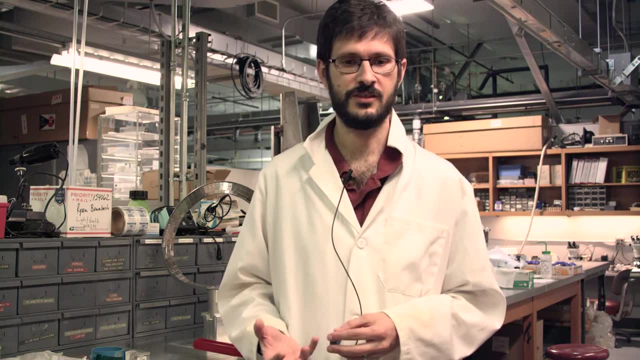 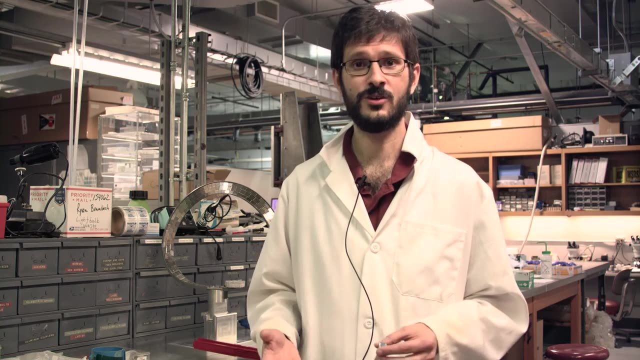 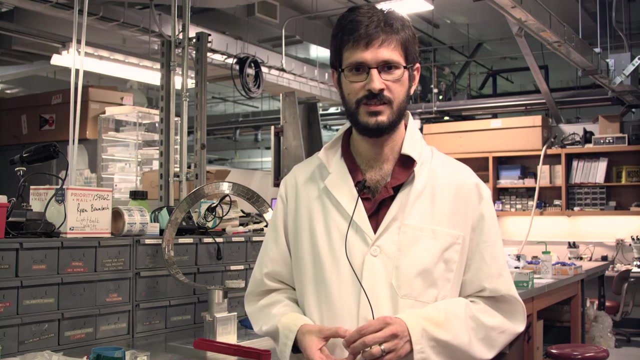 Conventional superconductors typically only work at very low temperatures, close to absolute zero. There are these unconventional superconductors which operate at much higher temperatures And although we've done a lot of work to characterize them and to try to discover new ones, they actually are still at the cutting edge of science. 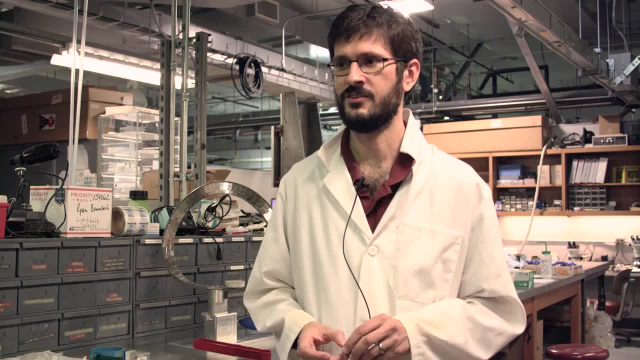 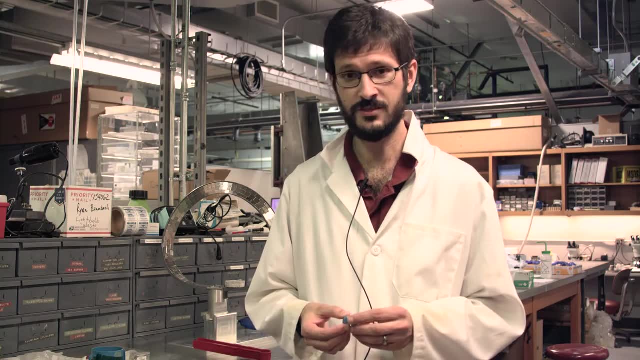 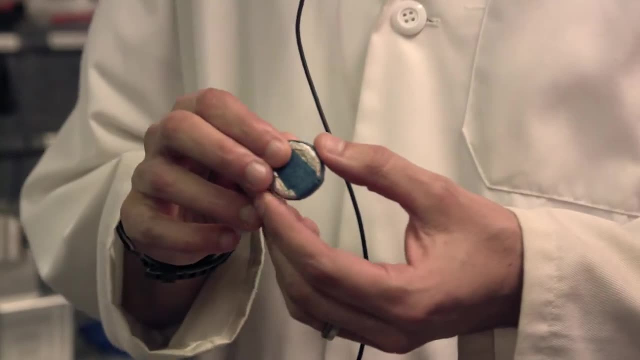 And one of the big efforts at the MAG lab is to try and understand the underlying physics of these types of materials. So what I want to show you now is a piece of yttrium barium copper oxide. So what's shown here is actually not a pure piece- well, a simple piece of the material. 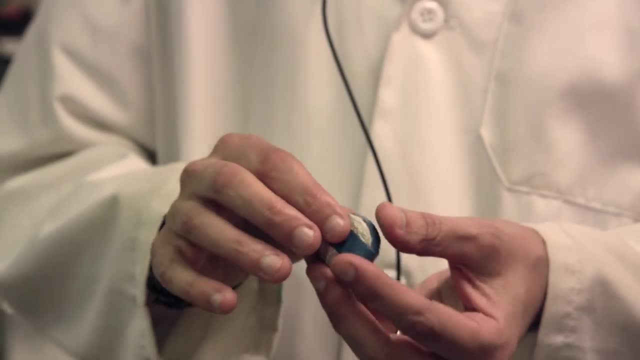 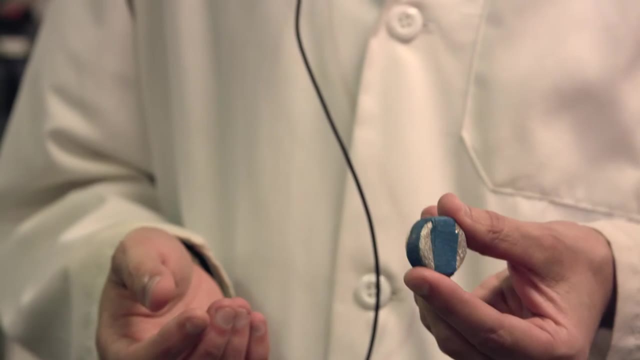 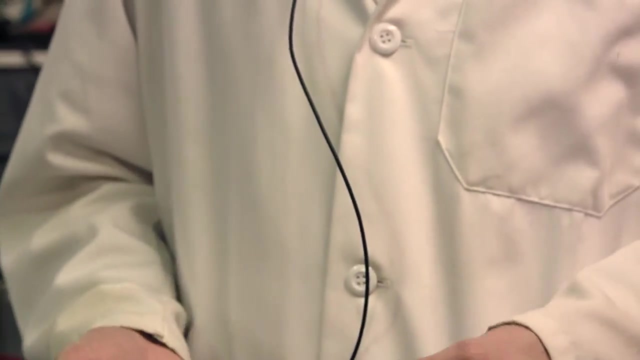 YBCO is a black crystalline material. What we've done here is we've wrapped it in aluminum foil to protect the pellet. This pellet was made here. It was made well, I don't remember- but either by middle school students or high school students. 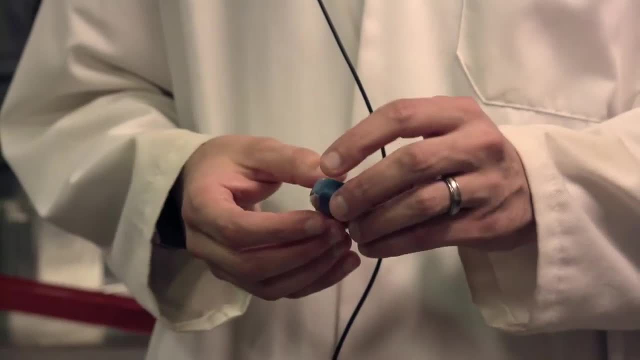 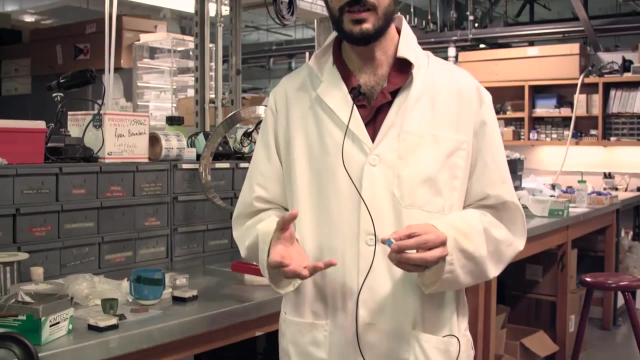 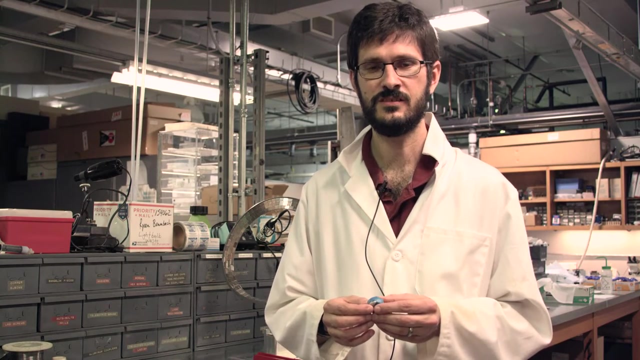 which tells you actually how accessible this is. And what I want to show you is one of the incredible properties that superconductors have, So I won't be able to show you this. Superconductors transmit electricity. They transmit energy without dissipating any energy. 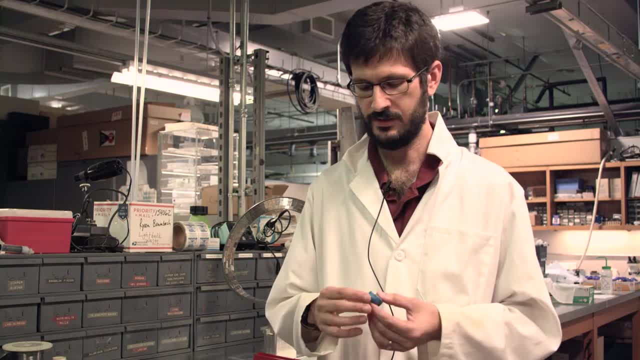 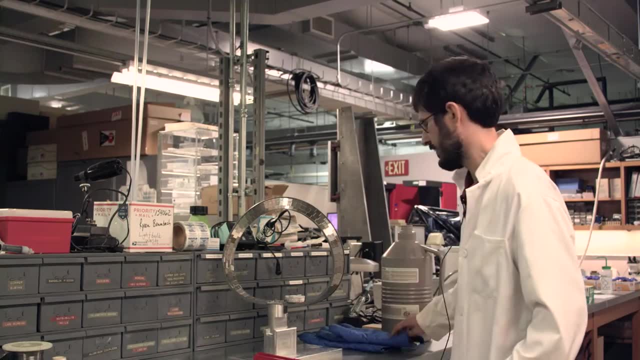 So, unlike your toaster, where when you run a current through it it heats up, if you run a current through a superconductor, it doesn't heat up. Superconductors do something else as well, and that is that they expel magnetic fields. 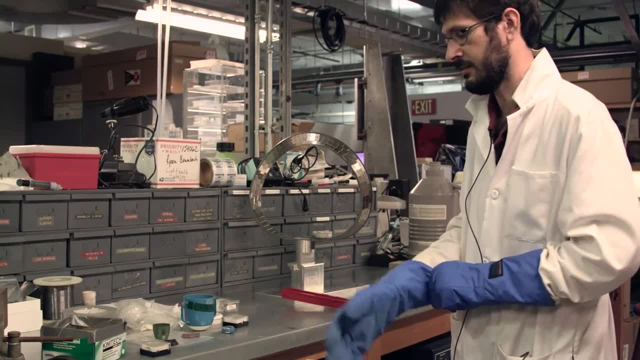 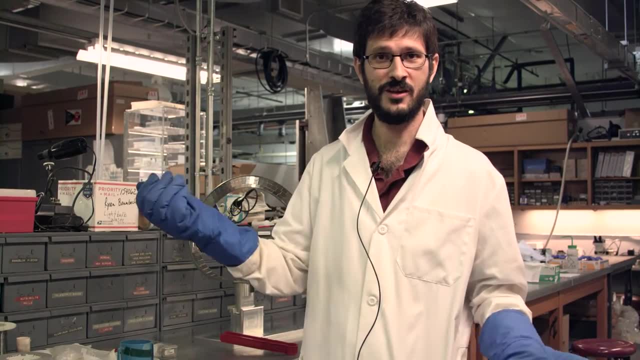 So in some sense they are a lot like a magnet. If you take two magnets and put them end to end, either they'll stick to each other or they'll repel. So a superconductor does something like that, but it's even more special than that. 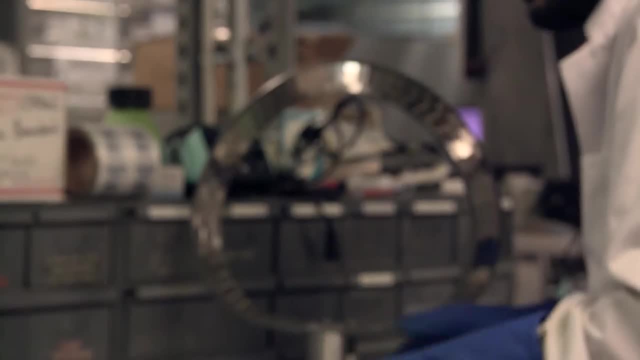 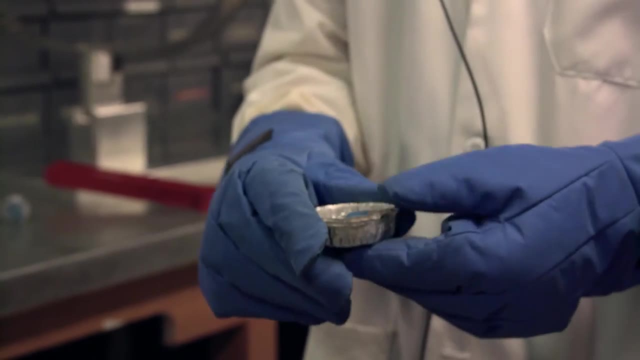 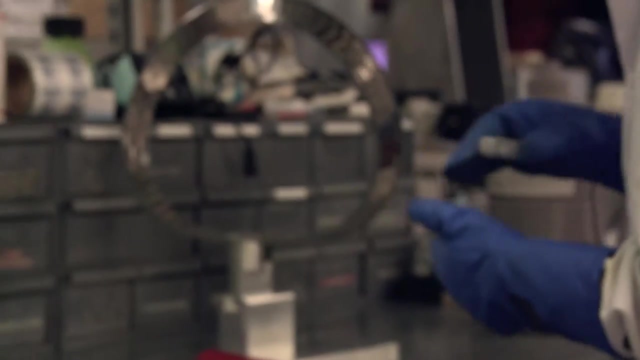 So let me show you something about this. So this is our piece of superconducting material. I'm going to put it in this tray and then I'm going to fill this up with some liquid nitrogen, which is a very cold liquid. 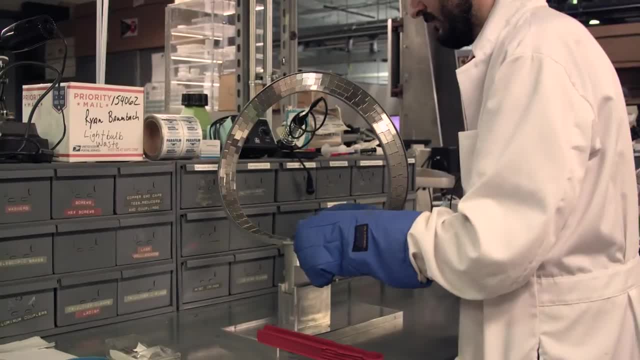 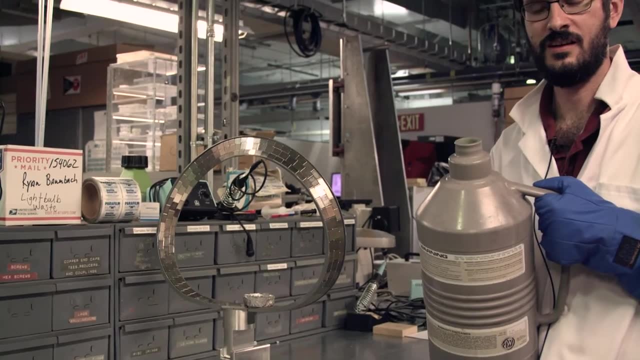 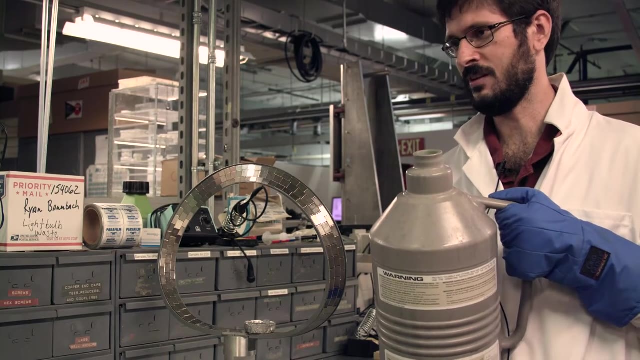 So let me put this here And I'll show you first. The liquid nitrogen can be a liquid when it's contained inside of, basically a giant thermos. Compared to the liquid nitrogen, a room temperature is very hot. So if I pour this out on the table, it'll vaporize immediately. 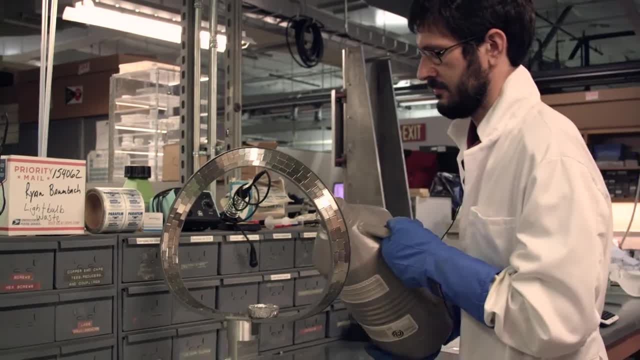 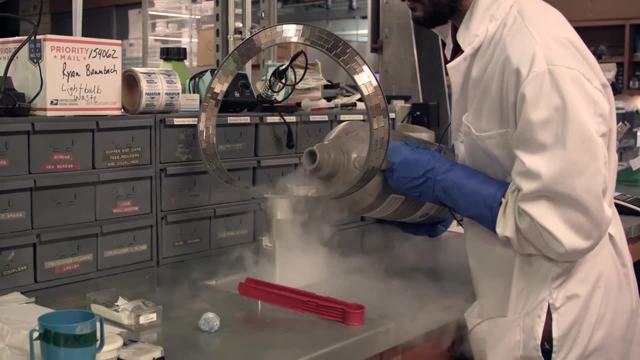 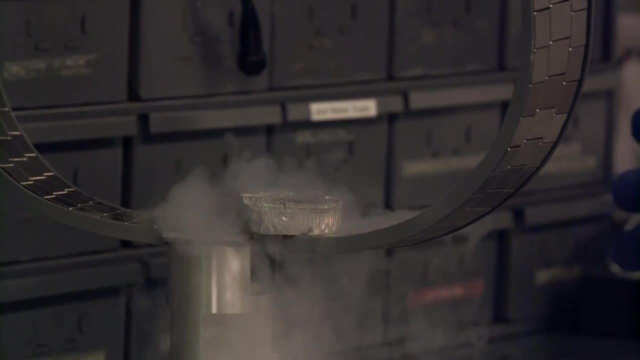 And that's what you'll partly see here. You can see that it is boiling. That's because this metal surface is extremely hot compared to the very cold liquid nitrogen. This is very similar to what you would see if you had a hot stove and you poured water on it. 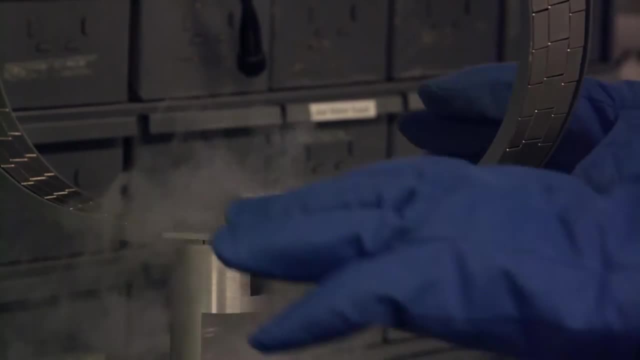 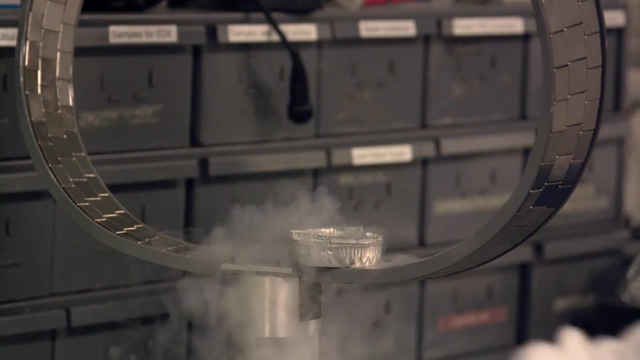 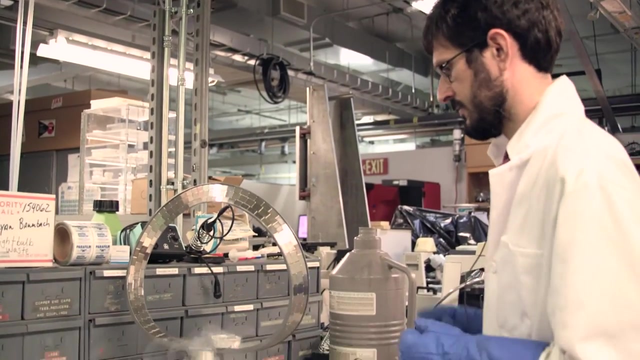 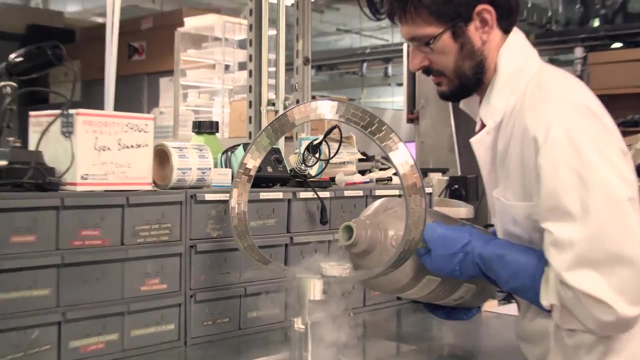 It's going to start to vaporize immediately. We also see sort of a mist coming off of this And at least partly that's some condensation coming out of the air. Some of it's liquid nitrogen boiling off too Okay, so it takes a little bit of effort to cool down the superconducting puck. 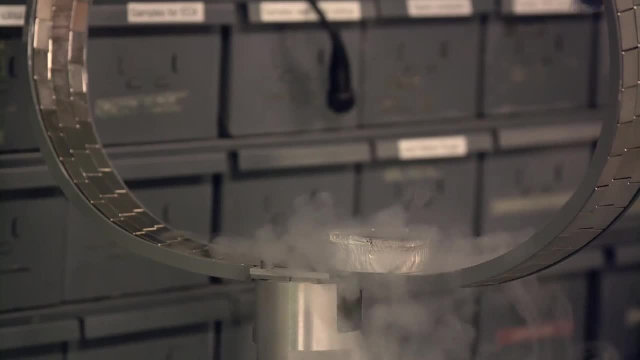 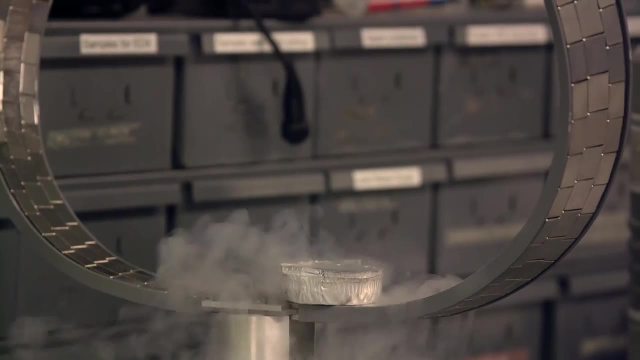 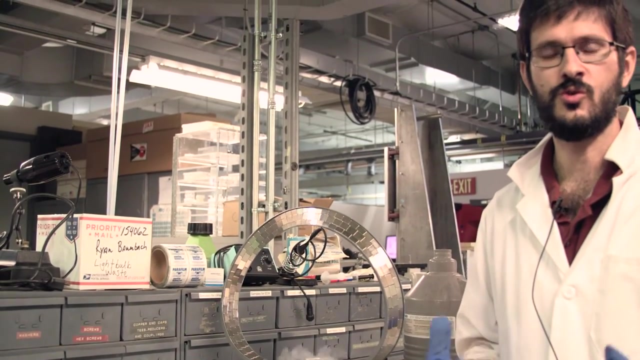 And as I cool it, the electrons that are in this material are undergoing a transformation from being sort of behaving like regular electrons in a piece of metal like the tabletop here, to entering a new quantum state that is completely unlike anything that we experience in our day-to-day lives. 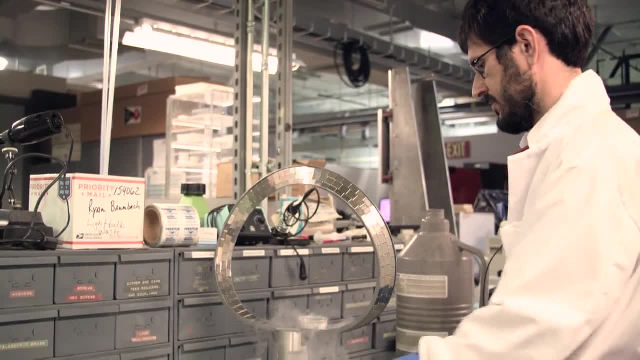 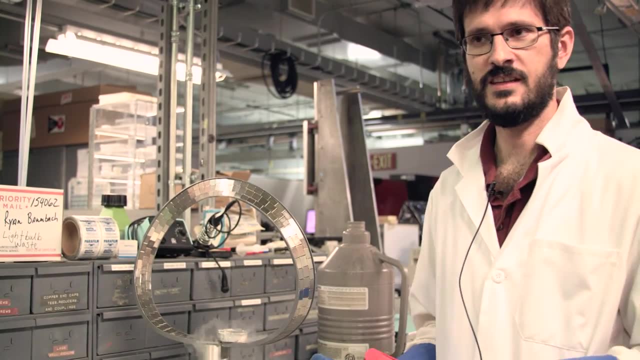 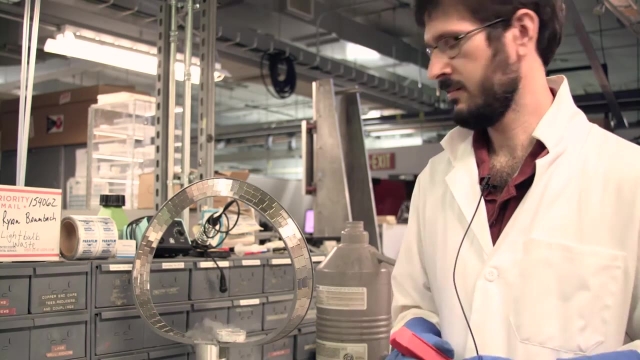 And that quantum state is called superconductivity. Alright, so I said, when electrons are in a superconducting state, they have two main properties. One is that they can go through the material without dissipating any energy, so they don't heat up that material as they move through it. 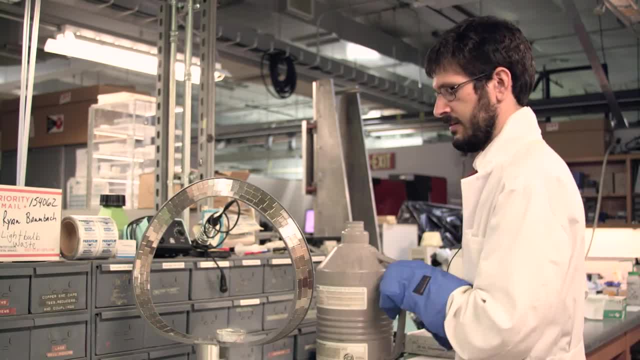 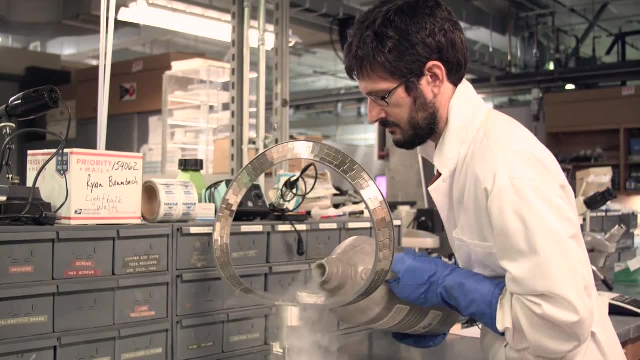 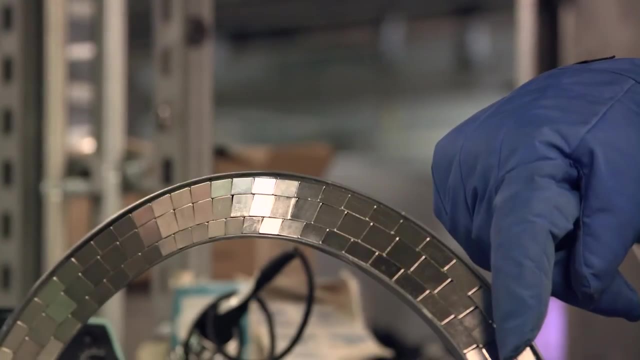 The other is that magnetic fields are expelled from the material. They're expelled from the bulk of the piece of superconducting material. I'll just put a little bit more on here. So what is on this track is a bunch of rare earth magnets. 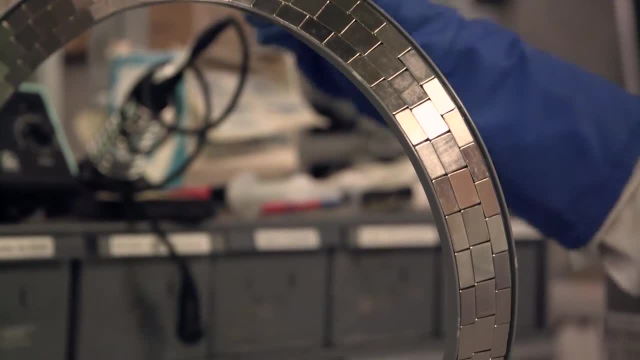 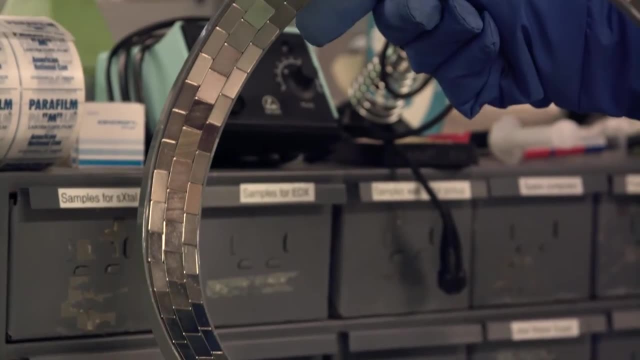 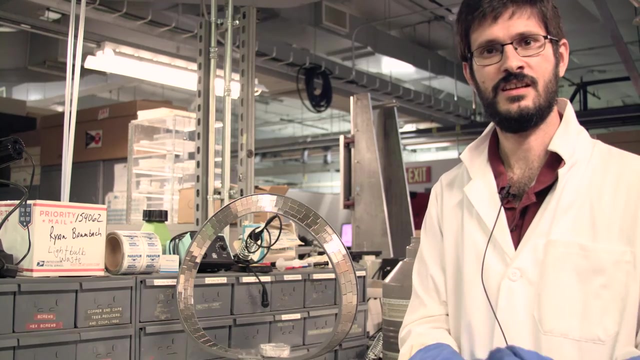 And they're held in place by a twisted piece of steel. Just for fun. the name of this shape is a Mobius strip, And anyone can make one of these If you just take like a strip of paper and put one twist in it and then connect the ends. 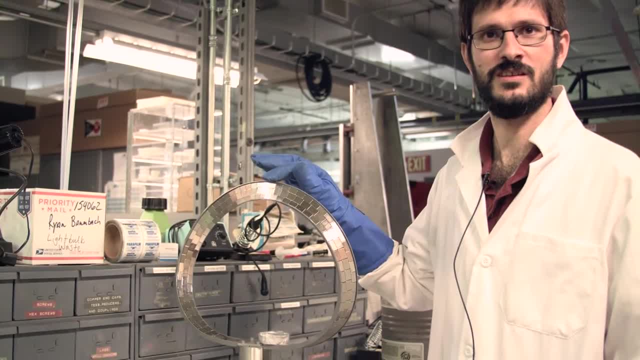 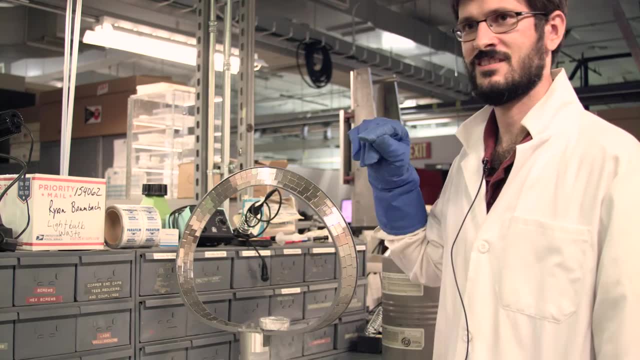 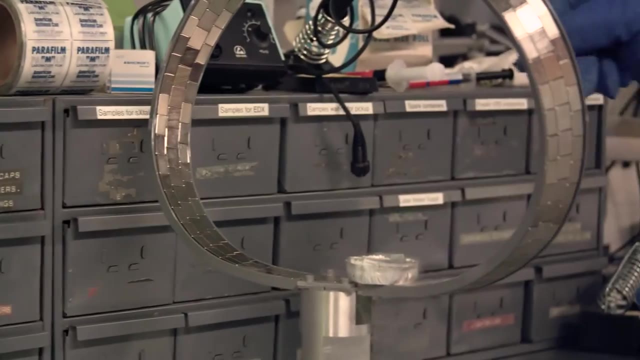 And it's a special shape that actually only has one side to it. So this is different from a piece of paper where you make a loop and it has two distinct sides. In a shape like this, both sides are connected to each other. Okay, so I said that the superconductor will expel a magnetic field. 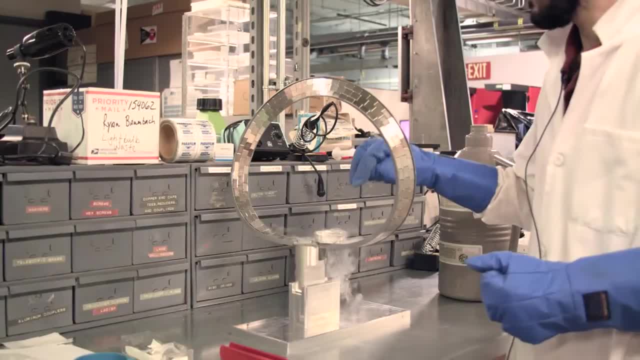 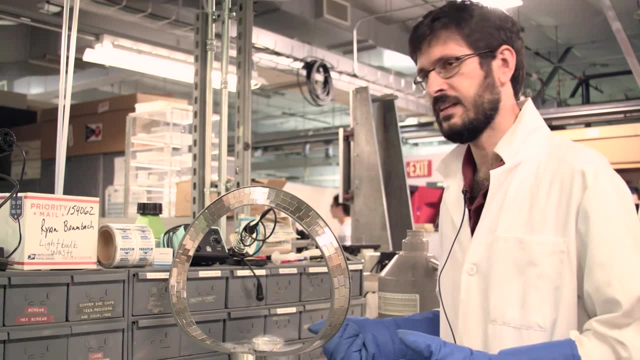 That means that they should repel each other. But the superconductor actually has one other property- Because it's what's called a Type II superconductor- And that is that it actually lets a little bit of the magnetic field that's coming out of these magnets. 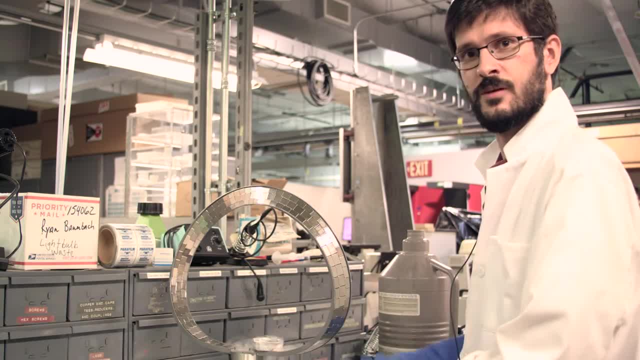 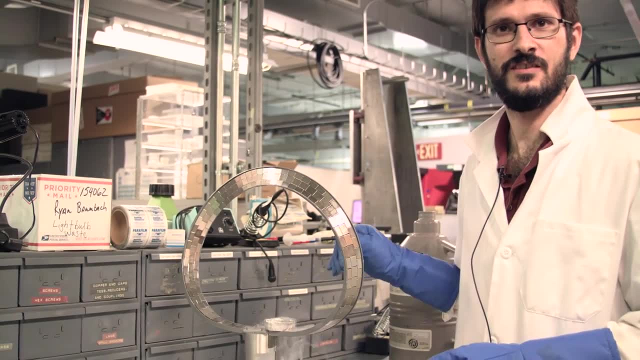 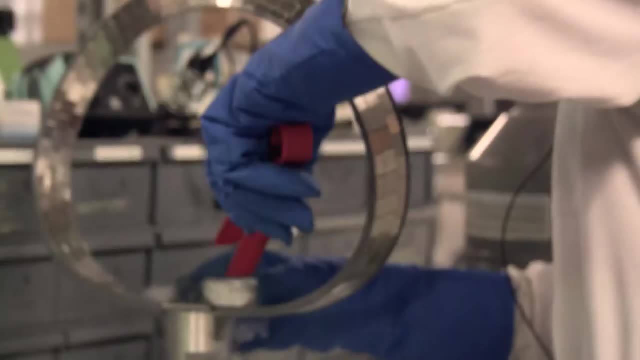 You can imagine, the magnetic field is coming out, sort of as loops coming out here, And those lines of magnetic field get trapped or pinned inside of the superconductor So they sort of act like springs to hold it in place. So let's see what happens. 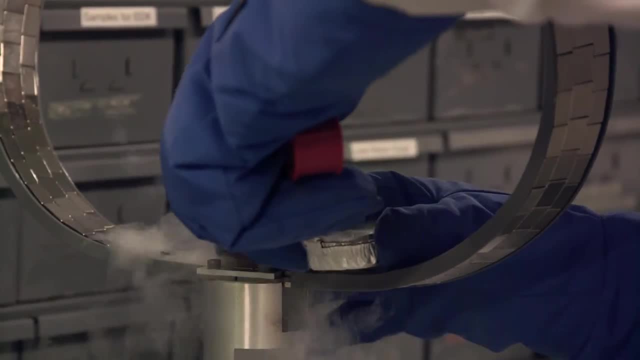 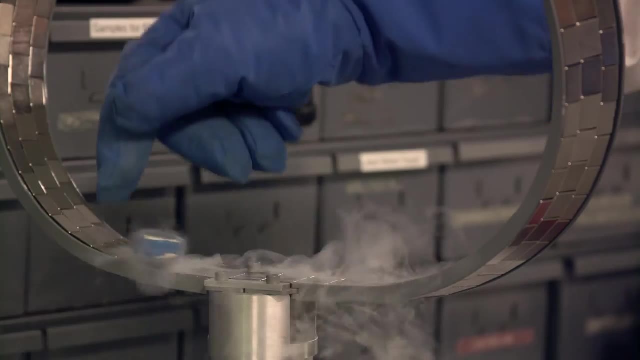 I'm going to pull this out of here. First of all, you can see that the magnet levitates, And not only that, but as it levitates it sort of holds on in place, Which is different from putting a regular magnet over this. 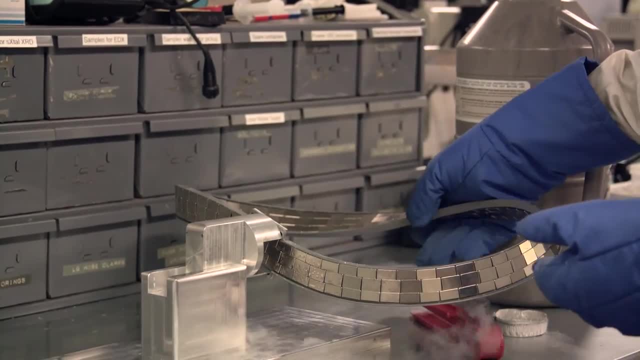 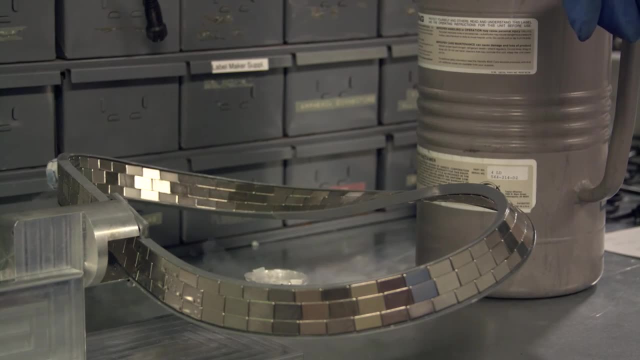 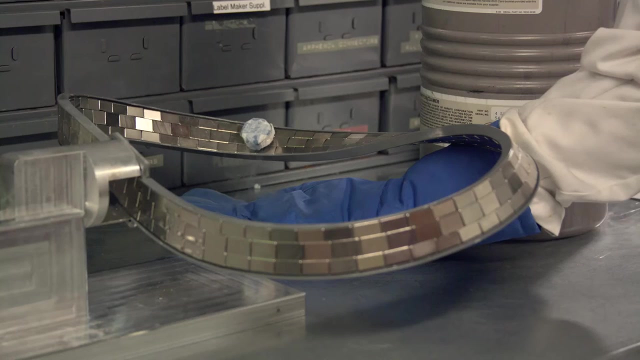 If I bring this down, you can see one of the interesting properties of the superconductor is that the magnetic field pins the superconductor in place. So you can see that as this goes around on the Mobius strip, it can hang from it, it can go from the side. 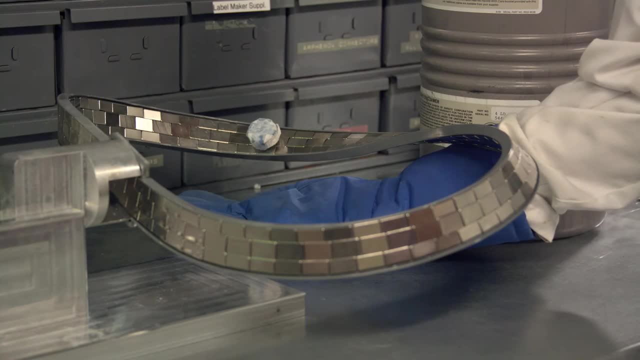 until the material warms up. So that's an important demonstration. actually, When the material warmed back up, it went back through its superconducting phase transition. The electrons in here stopped behaving as these special particles that have superconducting properties. 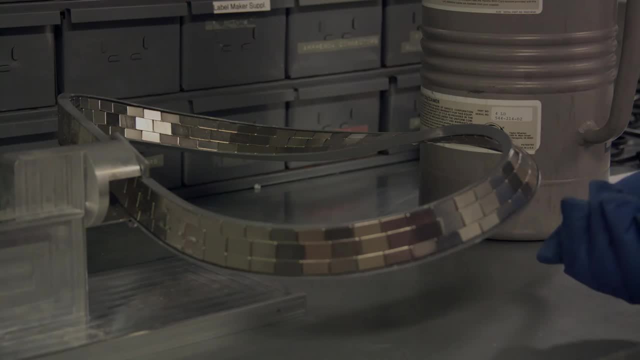 And began to again behave just like regular magnets, Electrons. 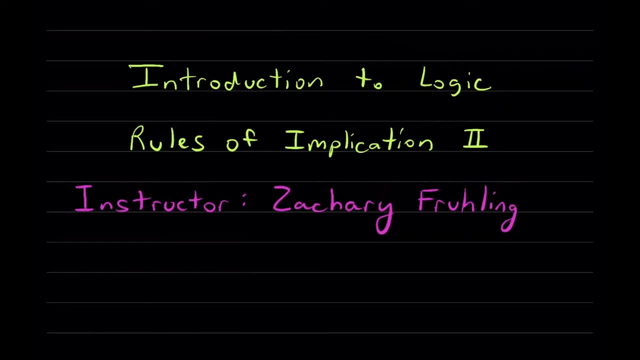 Hi everyone and welcome to week five of Introduction to Logic. This week we are going to be continuing our foray into the natural deduction proof method for propositional logic and we're going to be covering the second batch of implication rules from the Hurley Logic textbook. Now the first. 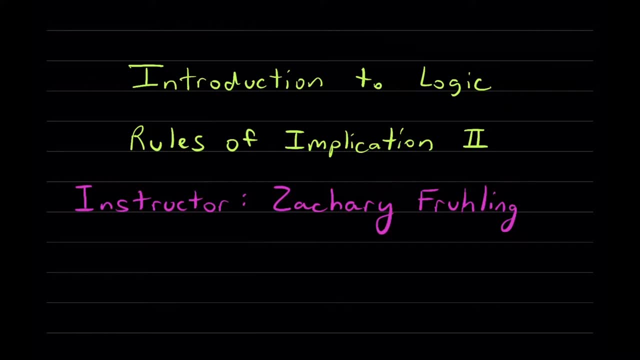 thing I want to say is that these new rules that you're going to learn today are in addition to the previous rules and, in general, this is going to be true. Week after week, you're going to learn a new batch of deduction rules, and those rules are cumulative. They're in addition to the rules. 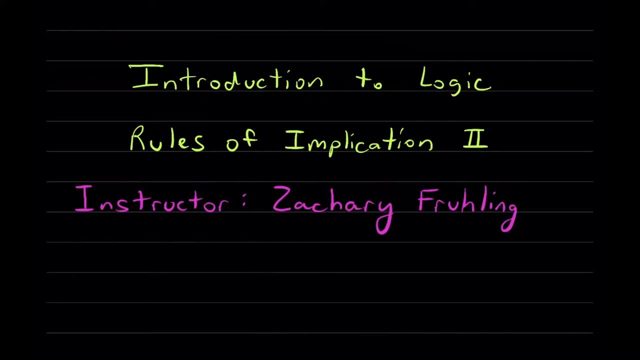 that you've learned previously. so our system of natural deduction rules is going to grow and grow and grow. So, without further ado, let's dive in to talk about the first rule of implication, first new rule of implication called simplification, abbreviated SIMP, And the rule basically works. 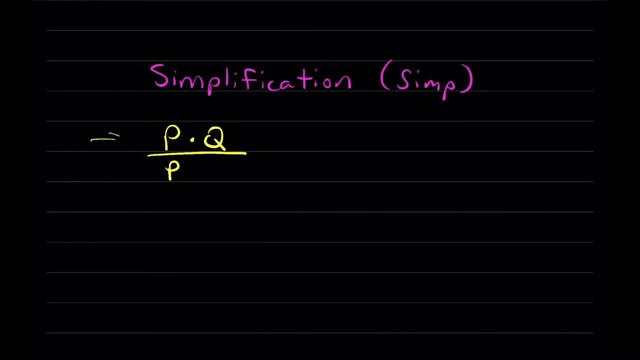 like this: If you have a conjunction on its own line, something like p dot q with a dot as the main operator, you can take the term on the left, the left hand conjunct and write that on its own line. And if you have a conjunction on its own line, something like p dot q with a dot as the line. And if you have a conjunction on its own line, something like p dot q with a dot as the main operator, you can take the term on the left, the left hand conjunct and write that on its own line. And if you have a conjunction on its own line, something like p dot q with a dot as the